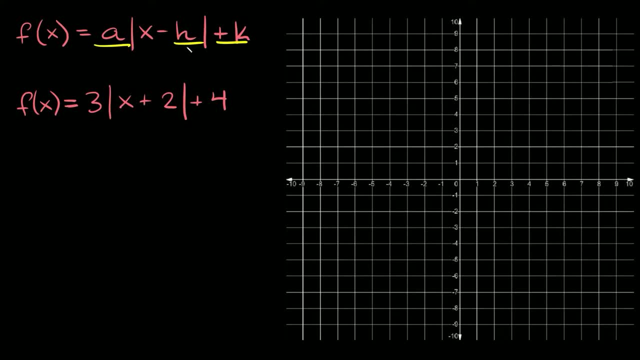 here. give you the vertex of your graph. So then h and k. the vertex would be at, basically h comma k. So the h is basically your x and the k is your y. Okay, those are literally the only two things you need to know in order to graph an absolute value function, right? So let's start with a more. 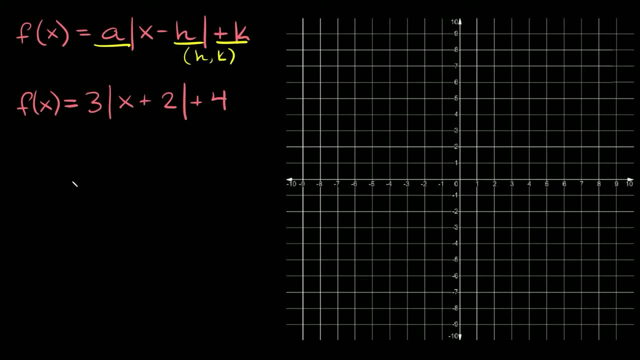 complicated one, and then we're going to do some easier ones. so you see how they all actually do tie in together. So here we have: f of x is equal to three times in the absolute value, bars x plus two, and then a plus three times in the absolute value: bars x plus two, and then a plus three times. 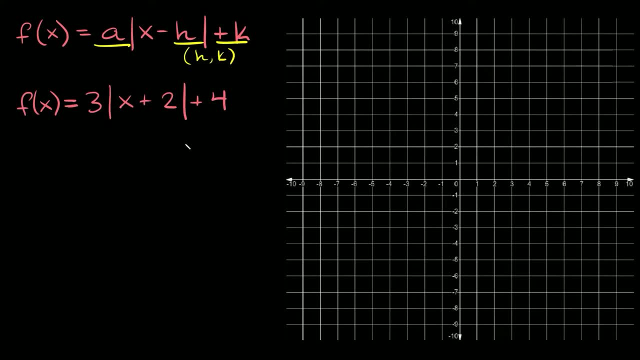 and then a plus three times in the absolute value bars x plus two, and then a plus three times in the absolute value bars x plus two, and then a plus three times in the absolute value bars x plus four on the outside. Okay, so again, the first thing you want to do is find your vertex and 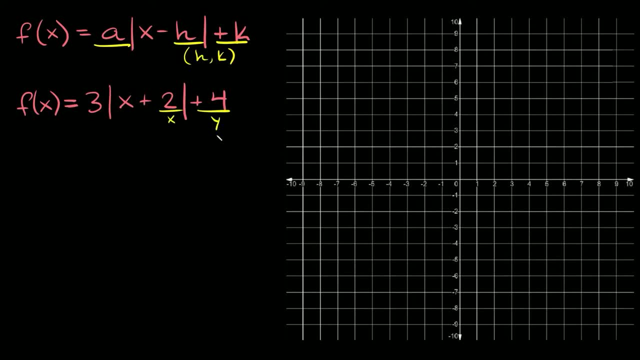 that comes from your h and your k right. This is your x and this is your y. The only difference is for your x term. you basically take the opposite sign. So here we have a positive two right. So for your x coordinate it's actually going to be a negative two, and then for your y, this still. 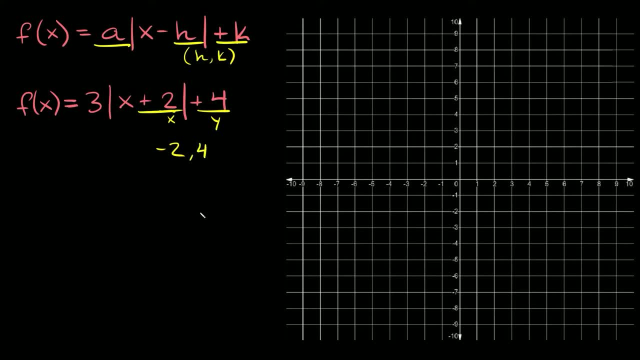 just stays the same. So this is positive four. so then your y stays as positive four. So the y is negative. two comma four, right. So then we'll go negative. two comma four, right there. Okay. so this is negative two comma four, right there. And then the other thing is your slope, all right, So. 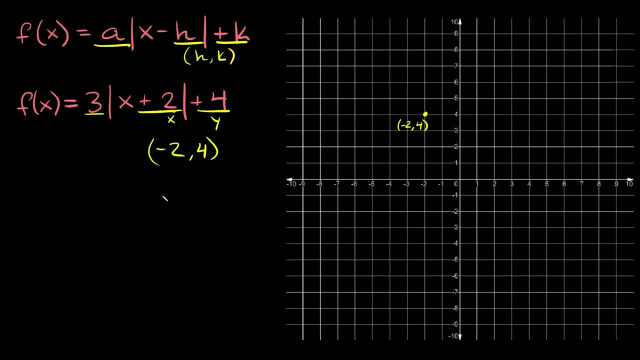 this number out here in front gives you the slope of your graph, because an absolute value function, basically, is shaped like a v. okay, Or it is shaped like a v, So in this case it's telling us that the slope is three. Okay, so, starting at the vertex, if we know our slope is three, we're. 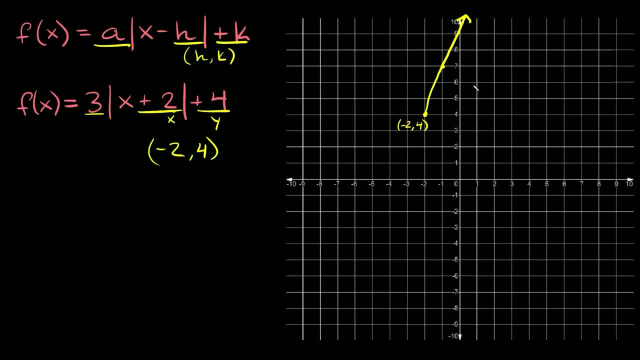 going to draw a straight line. So then there's your other point. All you do is draw a straight line, okay, But remember I told you that the absolute value functions are v-shaped, so we need this side also. So again, we're going to go up one, two, three, but then we're going to go over one. 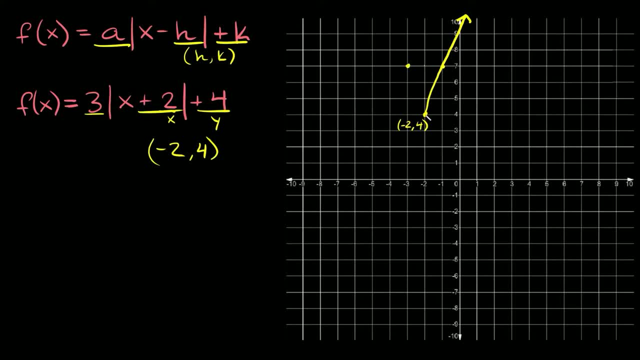 to this side, right? So then we know our other point is right there. And then you just draw a straight line, just like that, okay, So then the slope of this line over here, right, The slope is equal to three. and then the slope of this line is basically equal to negative three, okay, And 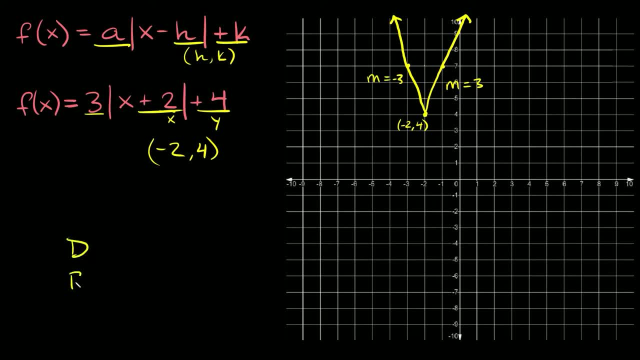 that's literally all there is to it. Now we just need to find the domain and the range. So the domain is our x value limits, right side to side, and then the range goes up and down our y value limits. So for the domain, you can see that the graph is going to go forever. basically, in that, 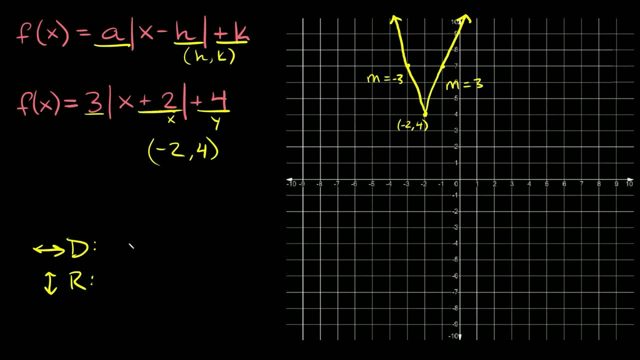 direction towards negative infinity and in that direction, towards positive infinity. So the domain is all real numbers and that's the symbol for all real numbers. And then the range. our limits for the range are basically from positive four to positive infinity. right, Because the graph just goes up. 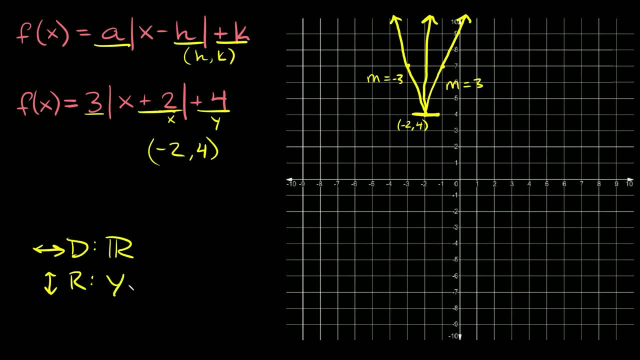 So then here we could say that the range is y is greater than or equal to positive four. okay, So hopefully not too bad, Let's just try a few more. Okay, so here's basically the same equation. The only thing I did is change the slope from positive three to negative three. okay, But 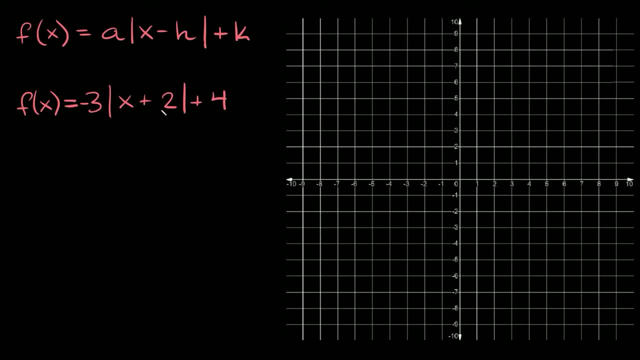 in any case, let's just use the two things we need, right? So all we need is the vertex. So we know the vertex is at these two numbers, right. So we know the vertex is at these two numbers right here. And you just want to take the opposite sign, right? So it's at negative two comma four. 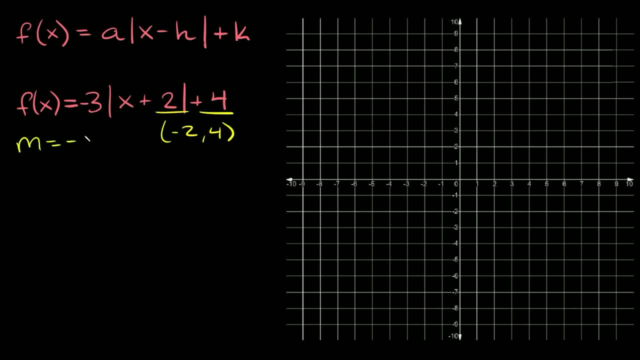 And then in this case the slope is equal to negative three, right. So again the vertex is at negative two comma four. And then now the slope is negative three, right. So this time we're going to go down one, two, three and then over one. Okay, so our slope right here is at negative two. 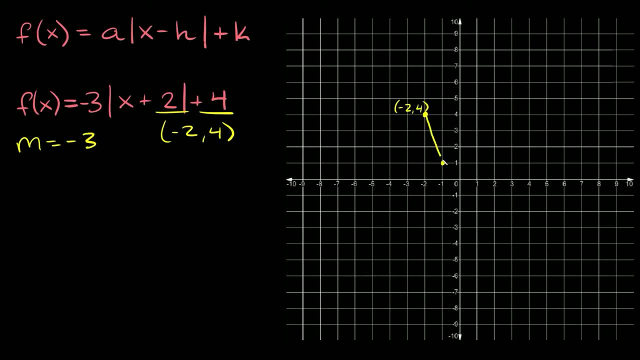 four. and then we went down at a slope of negative three, And then we went down at a slope of negative three, like that right. and then we're going to do the same thing in the other direction. so we have our v shape. so we went down three over one. so we're going to go down three and over one in this. 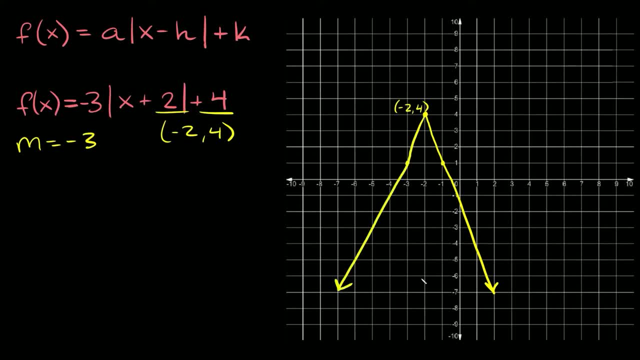 direction this time right. so then we'll draw our line right there, okay? so then there's our absolute value function and then again the domain and the range. the domain is basically always going to be the same thing here. it's going to be all real numbers, and then the range, this time goes from: 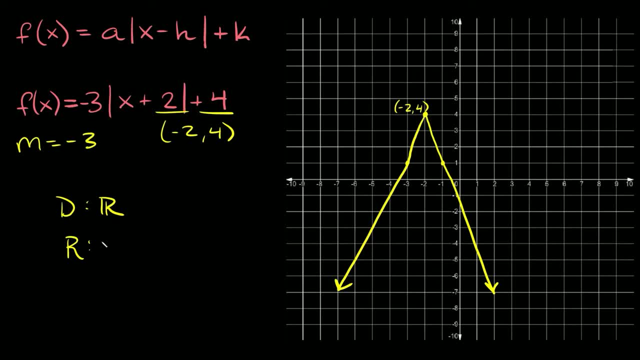 positive four down towards negative infinity. right, so we're going to say that our y values are less than or smaller than or equal to positive four. okay, so here we have. f of x is equal to the absolute value of x minus three. okay, so a couple things you might notice right off the bat is we're 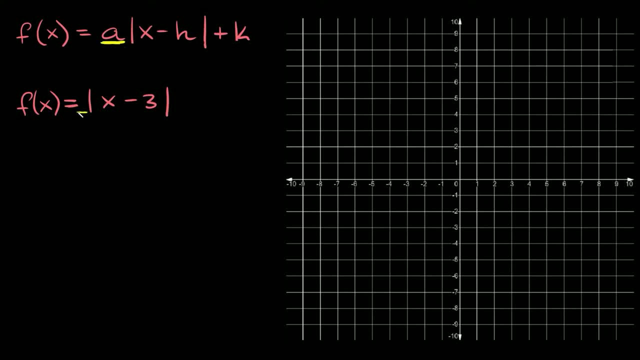 missing, basically our number, our a term right here, right in front, right, and whenever you don't see a number right there, that means there's basically a, an invisible coefficient of positive one. okay, so we're going to draw our line right here and then we're going to draw our line right here. 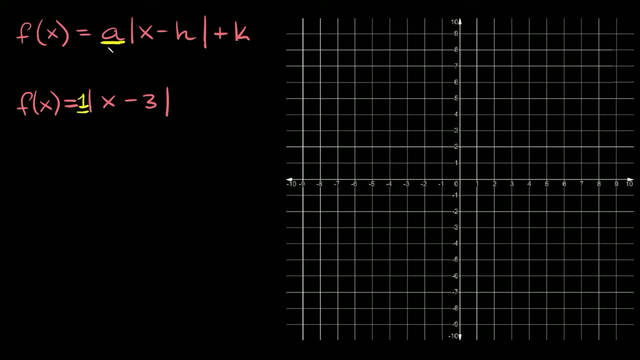 okay, so in this case you can basically just plug in a one right there for a just, if that helps for for the slope purposes, and then here you can see we don't have a plus number at the end, right, we don't have our plus k, so you can imagine this as putting plus zero. okay, same exact thing. so if you 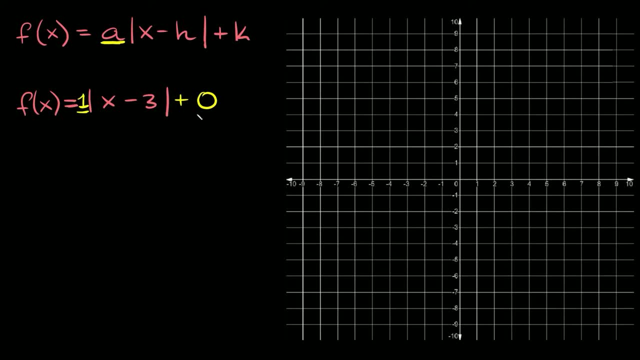 want to fill in the blanks that way, just to make it a little bit easier. i highly recommend that, okay, because now it's going to be a little easier to pick out what we need. so again for the vertex, it's these two numbers, right, this one and this one. so just take the opposite. 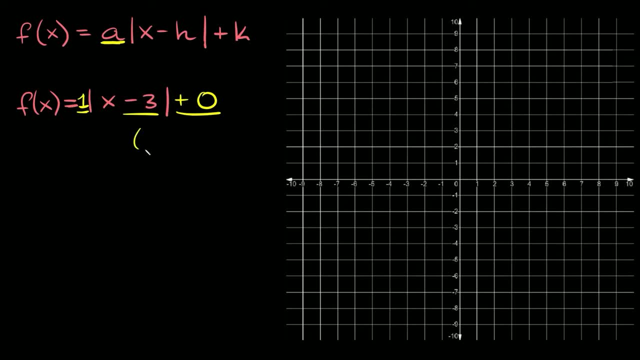 sign. so here we have a minus three, so that means for our vertex it's going to be a positive three. and then here we just have a zero, so it's a zero, okay. and then in this case we're going to have a slope of just positive one, okay. so again, the vertex is at three zero. so three zeros right there. 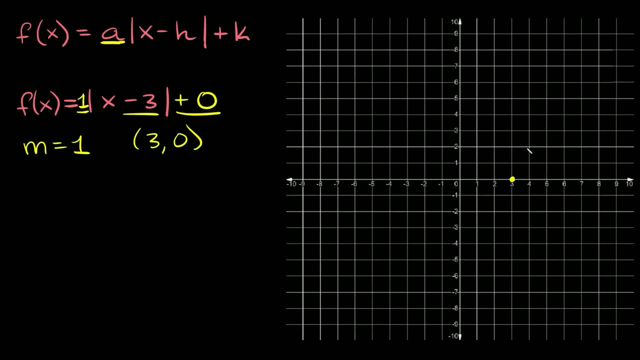 and then just a slope of one right. so, basically, up one over one, up one over one, up one right. so we'll just put one right there and draw a straight line like that and then, to complete our v, we'll go in the opposite direction, right so? 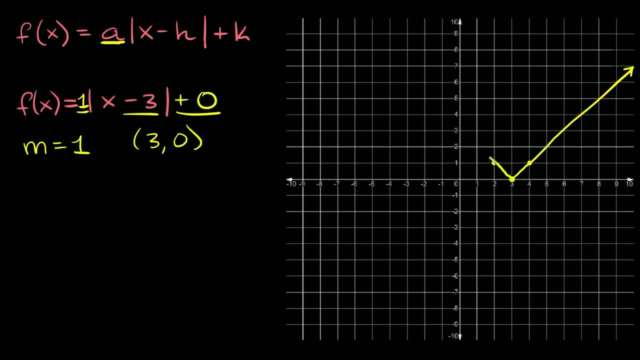 we'll go up one over one, like that, and complete our B like that. boom, alright. so then the domain and range. again, god, these are fun. so the domain is gonna be all real numbers and for our range, our Y limit right here is at 0, and then it. 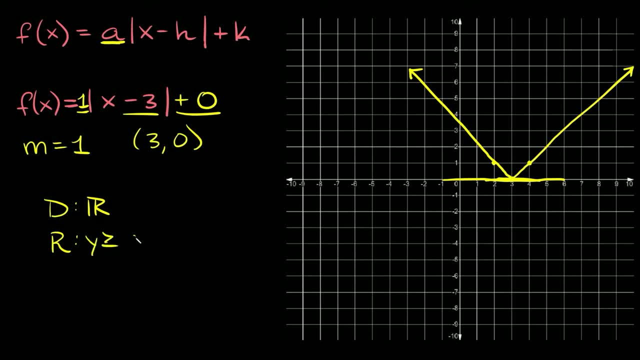 goes to positive infinity, right? so here Y is greater than or equal to 0. okay, so here we have. f of X is equal to the square square root, P, the absolute value of X plus 4. okay, so again you can see we don't have a number right here there's. 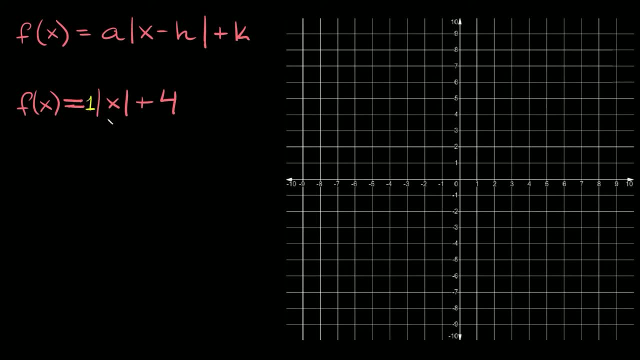 no a. so again, you can take that to be a positive 1, and we don't have another number inside the absolute value bars with the X, right? so really you can think of this as let's just write it out: f of X is equal to 1 times the absolute value. 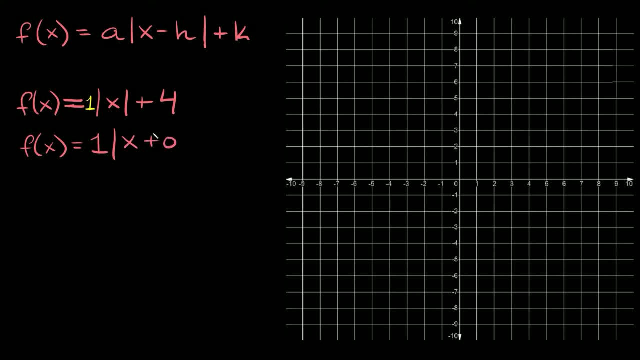 of X plus 0, right? since we don't have an actual number in here, just replace it with the absolute value of X plus 1, right? so here we have: f of X is equal to with 0, because it's the exact same thing. and then we have this plus 4 at. 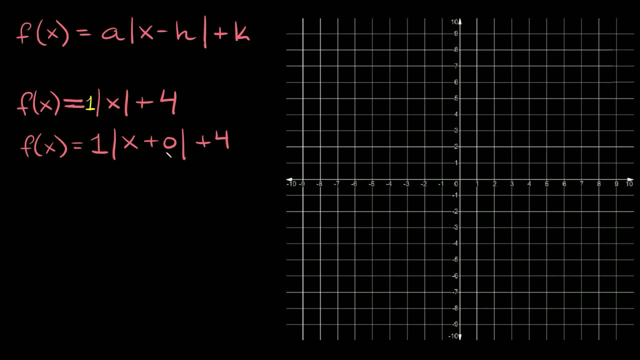 the end. okay, so then for your vertex it's gonna be at: well, 0 is not positive or negative, right, it's just 0. so the vertex is gonna be at 0 comma 4, and then the slope again is 1. okay, so 0, 4 is right. there there's the. 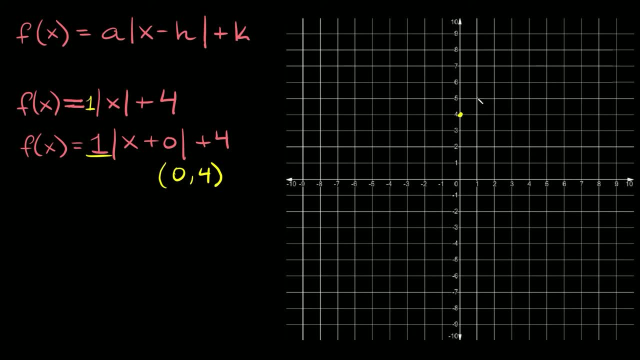 vertex and then the slope. it's just up: 1 over 1, right? so right there, draw a straight line. and then same thing in the other direction: up 1 over 1, right there, straight line, boom. okay. so there's your graph. and then the domain and range. 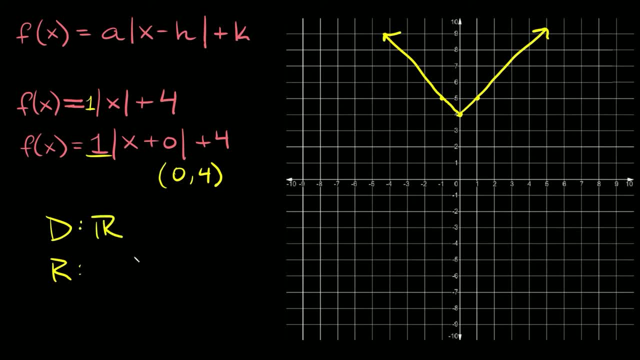 so the domain again is all real numbers, and then the range goes from positive 4 all the way to positive infinity, right? so we're gonna say Y is greater than or equal to positive 4. all right, here's the last one, and it's gonna be a little. 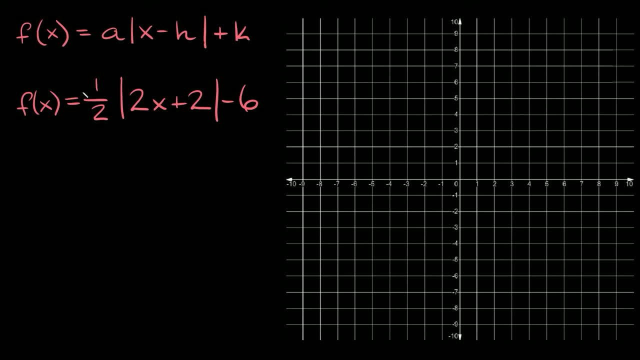 tricky because it's a little different from our form up here. so here we have: f of X is equal to 1 half, and then in a new form it's gonna be a little different from our form up here. so here we have, f of X is equal to 1 half, and then in a 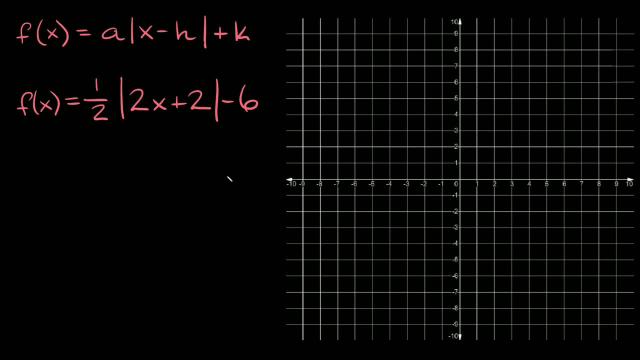 In absolute value: bars: 2x plus 2 minus 6 on the outside. Okay, so one thing that might stand out is that we have this extra coefficient next to the x, right, And we don't have that in our vertex form, right. 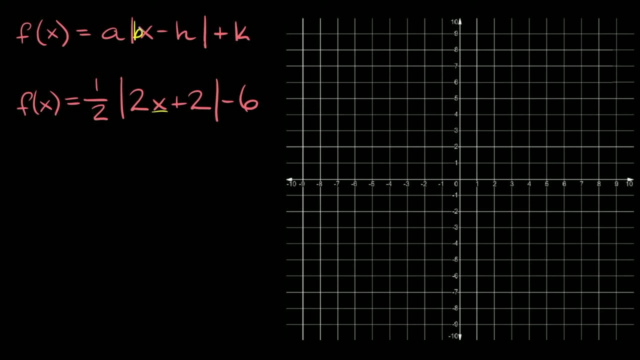 We don't have some number. let's just say b, right, It's not bx minus h, It's just x by itself, right, And here x is not by itself. We have this 2 attached to it, So to find the vertex it's not going to be as easy as just taking these last two numbers. okay, 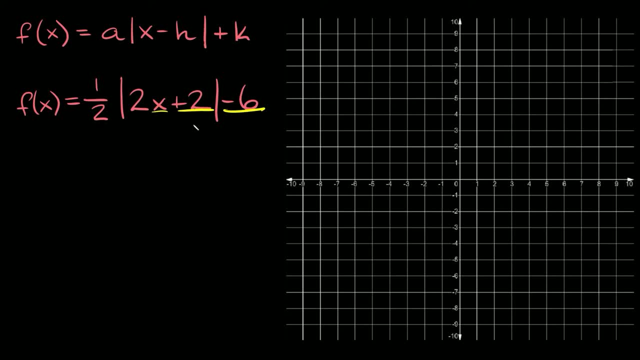 Well, it's actually going to be almost that easy, because this number is still going to be the same. It's just the x coordinate that's going to be a little different. So, in order to find the x coordinate, what you want to do is just take whatever is inside of your absolute value bars and set it equal to 0.. 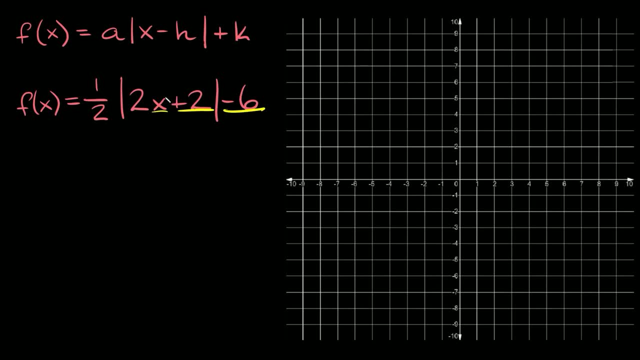 And that's basically what we've been doing this entire time. We've really just been setting what's in the absolute value, bars equal to 0, but I've just been showing you the shortcut way of doing it. But since we have this extra coefficient, we're going to have to just write it out. 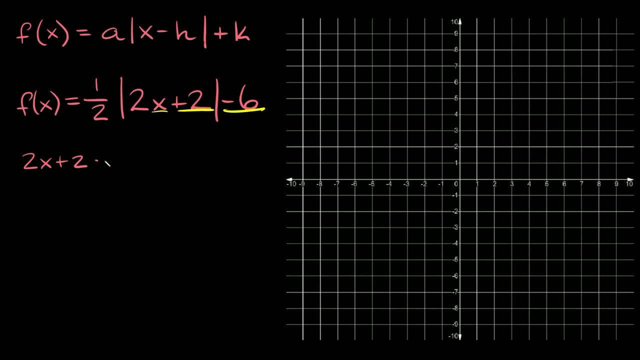 So here we have 2x plus 2.. So we're just going to set that equal to 0. And we're going to set that equal to 0. And we're going to set that equal to 0. And then just solve for x, okay. 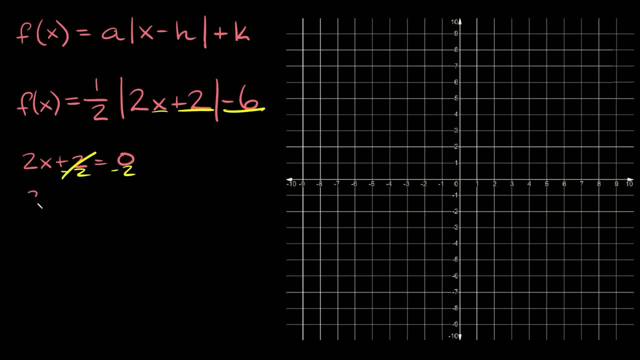 So here we'll subtract 2 from both sides. Those cancel out, So we get 2x is equal to negative 2.. Divide both sides by 2.. Those cancel out, So then we get x is equal to negative 2. divided by 2 is negative 1, okay. 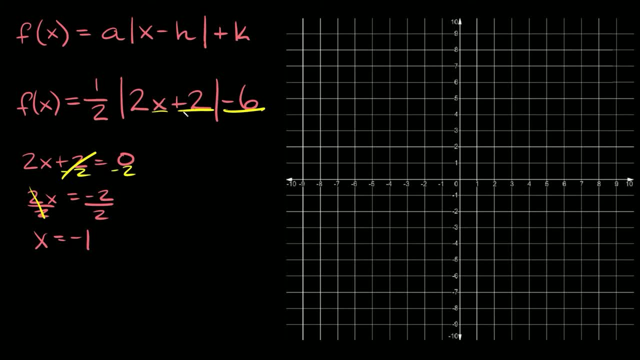 So then, in this case, the x coordinate for our vertex is going to be at negative 1.. So then it's going to be at negative 1.. And then this one is still the same, It's still just y. So we have minus 6 out here. 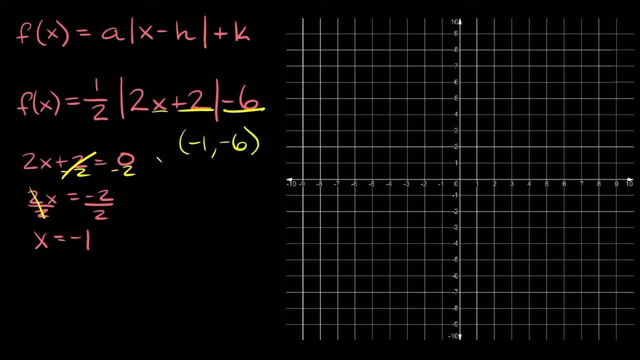 So it's still. So, it's still minus 6, like that, okay. And then the slope- same thing is also still the same. So the slope in this case is going to be equal to 1 half right? So let's plot our vertex at negative 1, negative 6.. 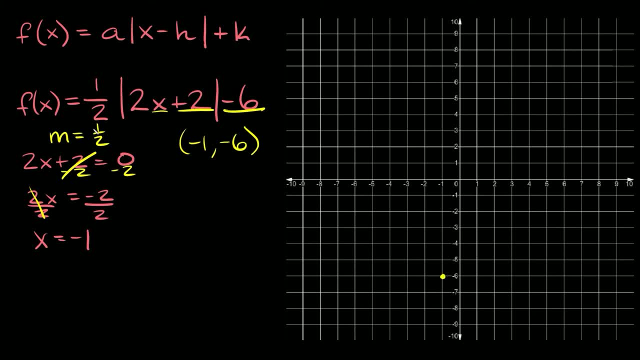 So negative 1, negative 6 is right there, And then our vertex is equal to 1 half, Or you can also count it as 1 over 2, right? So we'll go up 1 over 2, right. 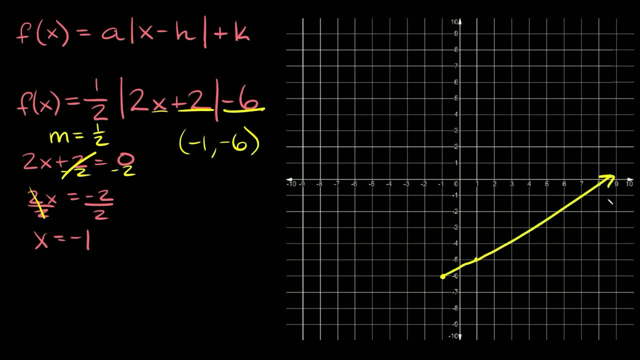 Up 1 over 2.. And so we'll connect the dots right there. And then same thing to the other side. We'll go up 1 over 2, right? So then connect the dots like so. okay, And there's your graph, right. 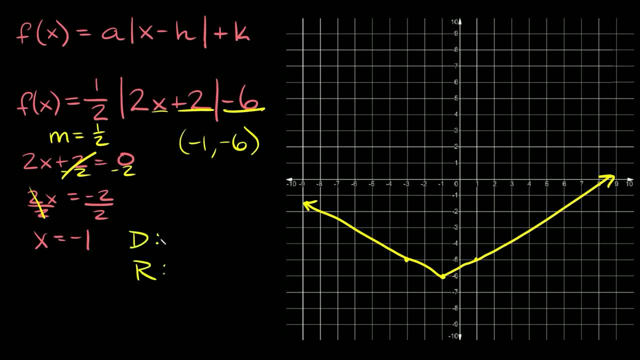 So the last thing we're going to do is just find the domain and range. The domain is all real numbers And then the range is from negative 6 to positive infinity, right? So we're going to say y is greater than or equal to negative 6..